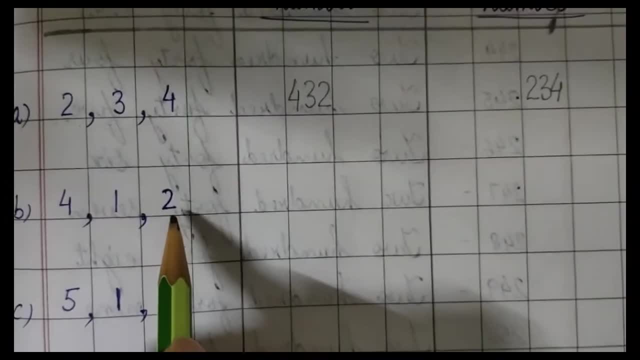 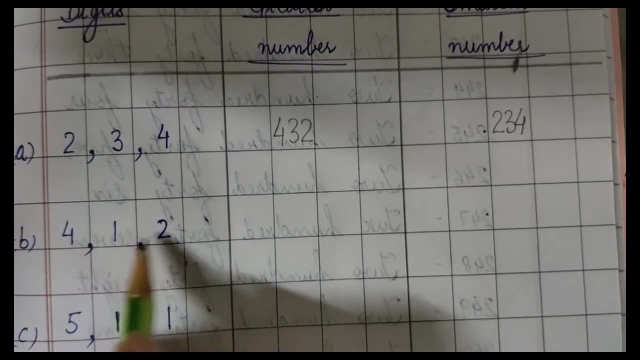 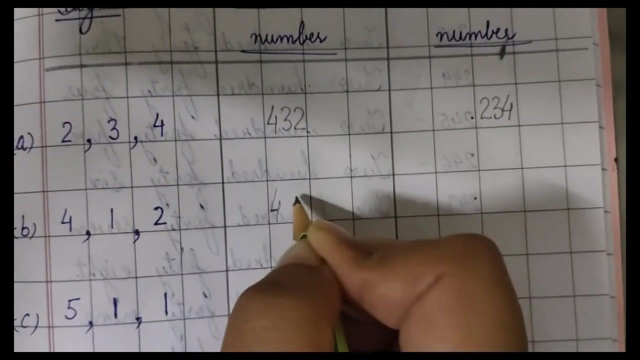 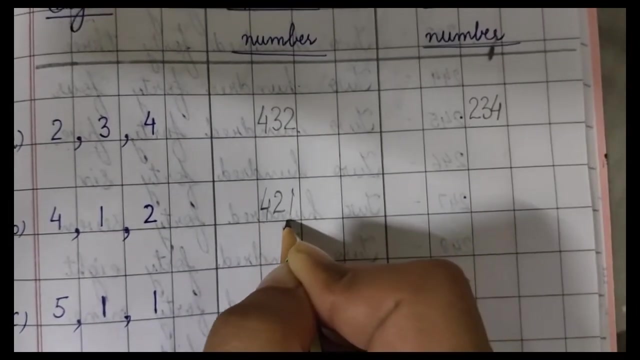 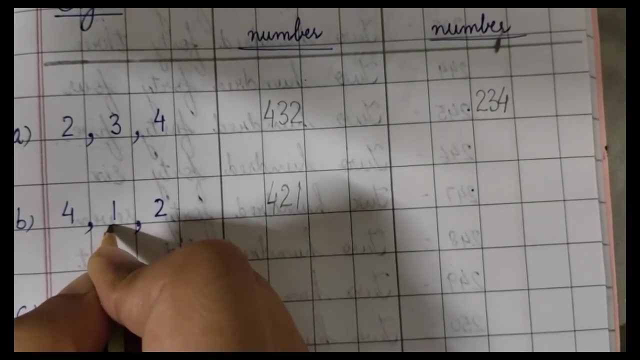 us see another one: 4, 3 and 4.. So how do we form the smallest number? We will arrange it in ascending order. with smaller number, 4, but simple number, The next iium number will be ridiculous. Arrange it in ascending order. 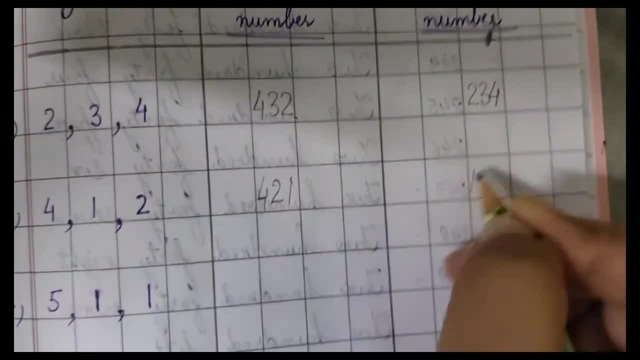 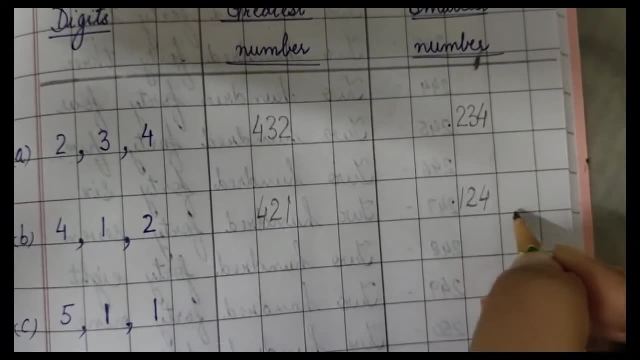 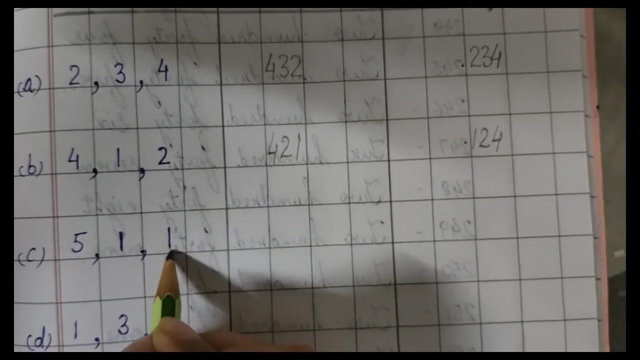 So smallest to biggest, 1, then 2 and then 4.. So smallest number will be 124.. Okay, students. Now next number is 511.. So how do we arrange to form greatest number? We will write the greatest number here. 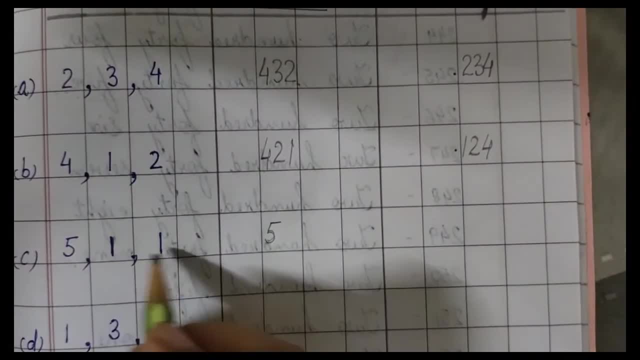 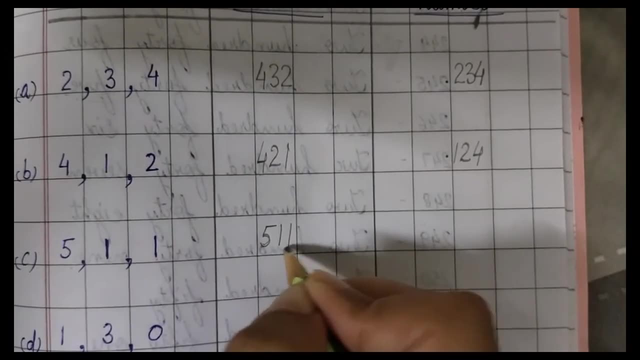 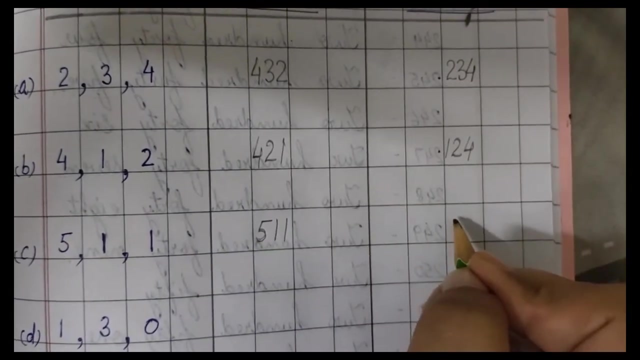 Greatest digit, that is 5.. And since both these are same, so we will write here 11.. So the greatest number will be 511.. And smallest number will be. the smallest number are 1 and 1.. So digits 1 and 1 are equal. 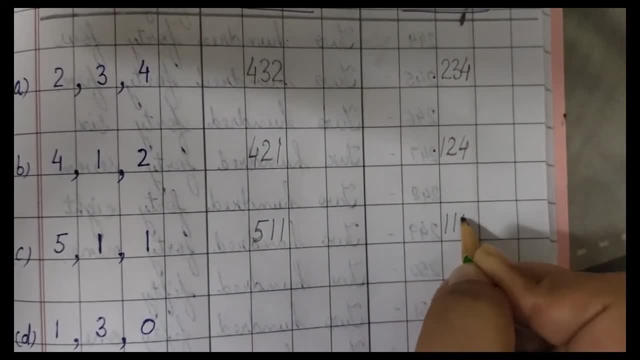 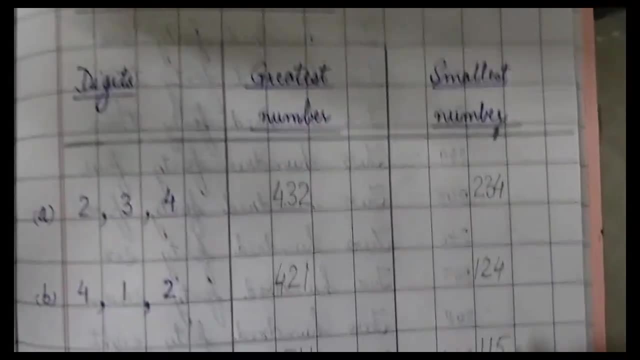 So these are the smallest. So we will write both the smallest digits And then we will write the biggest one, In ascending order. we have arranged it So 115 will be the smallest number. Okay, students. Now next number. 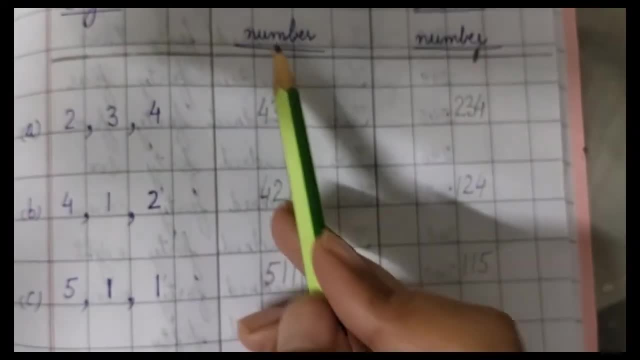 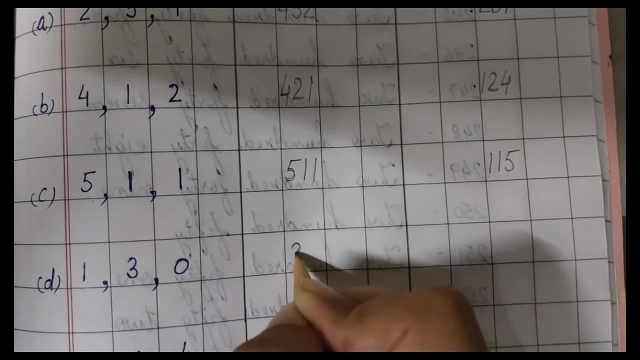 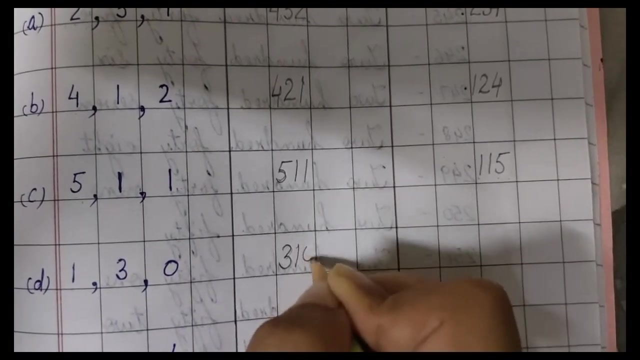 1, 3, 0. So how do we arrange it? in great arrange to form the greatest number, We will write the digits in descending order. So first number will be 3, then 1 and then 0.. 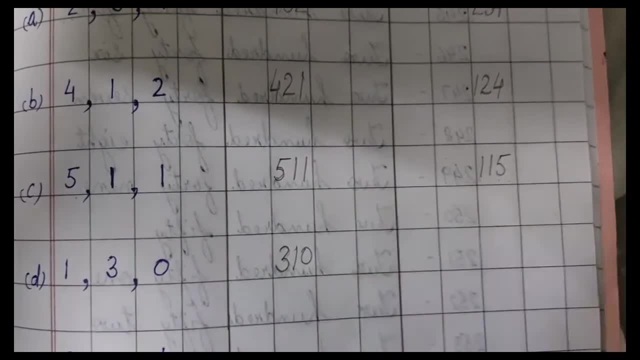 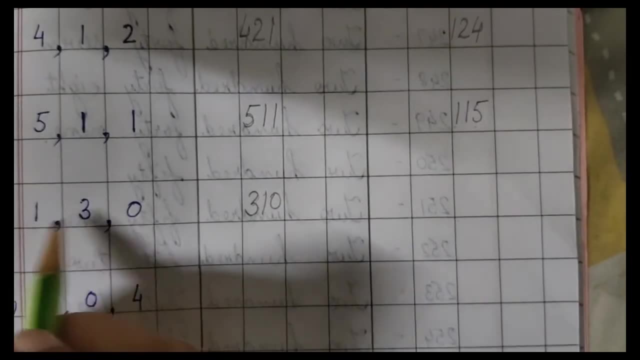 Okay, students. So 310 will be the greatest number, And what will be the smallest number? It will be 0.. 1, 3.. But no, it is wrong. So what do we get? 1,, 0, 3.. 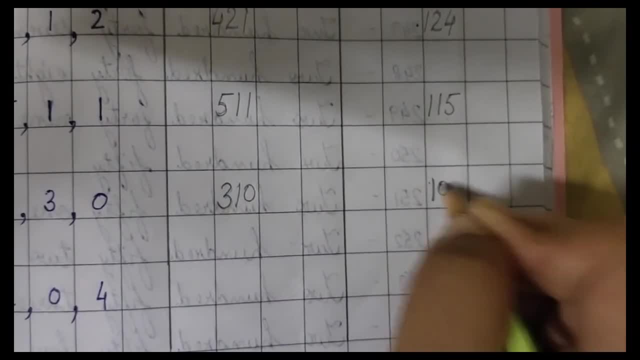 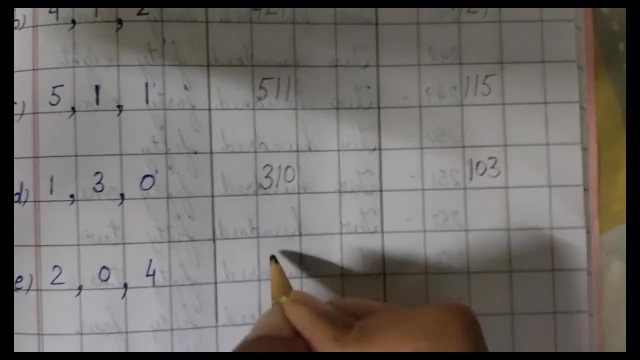 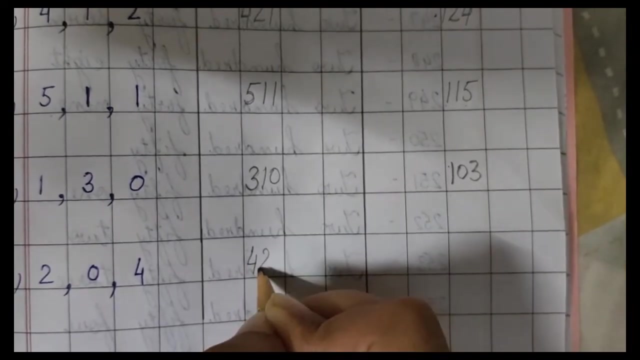 We will interchange that, So 1,, 0, 3 will be the smallest number. Okay, Last, 2,, 0,, 4 are the digits given. So what will be the greatest number? 4,, 2 and then 0..